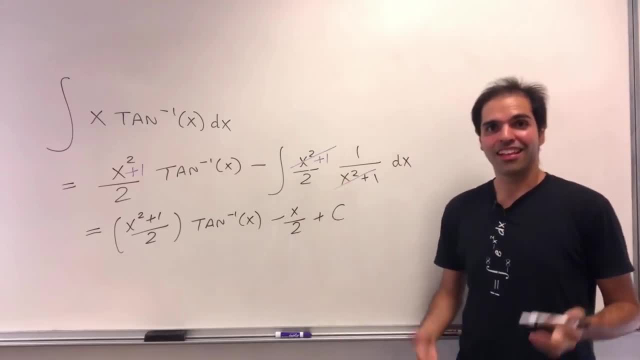 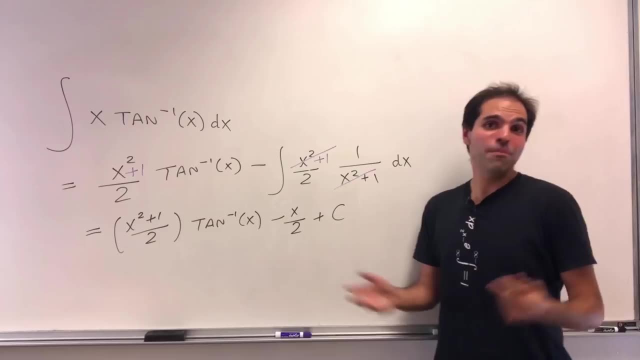 x over 2, plus a constant. That's it? Yes, that's it. Aren't you glad you found my video? Yeah, this is awesome Because, again, while your peers spend hours or minutes trying to solve this problem, you 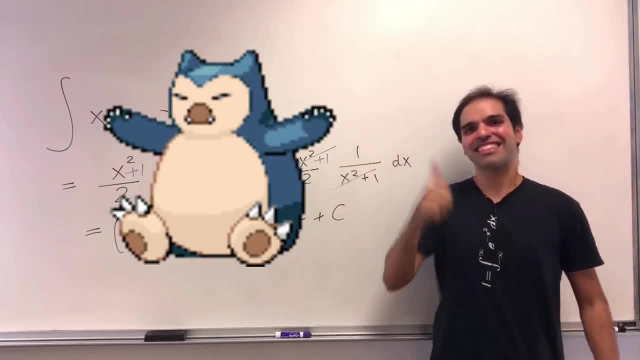 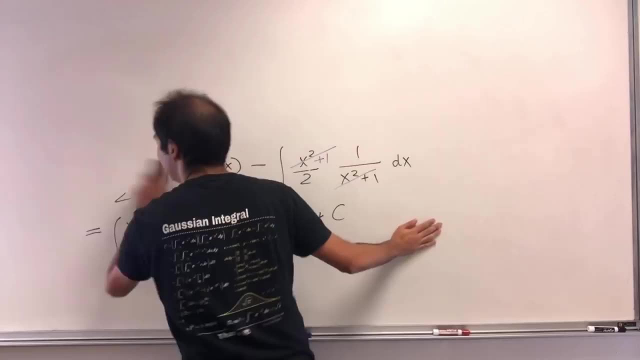 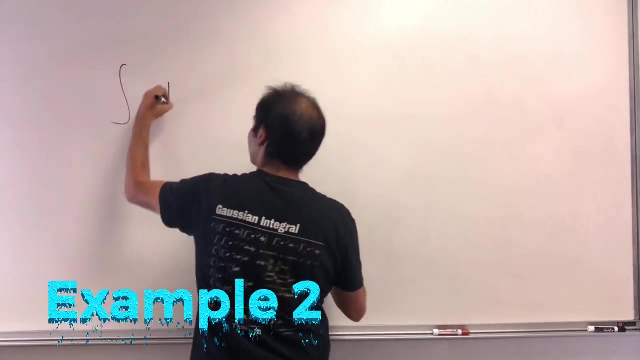 just do it in one minute and just relax. Awesome. And in fact, let me show you a couple more examples how to apply this. So, for example, speaking of ln degenerates, let's try to do the integral of ln of x plus. 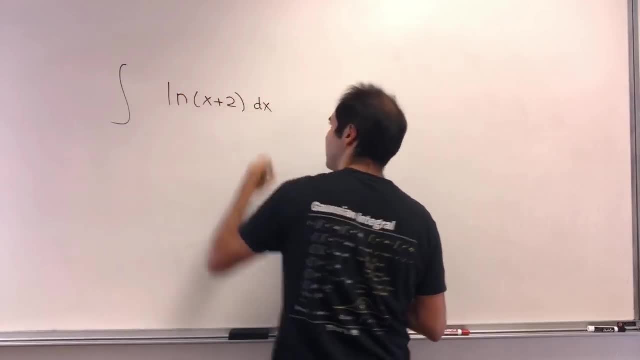 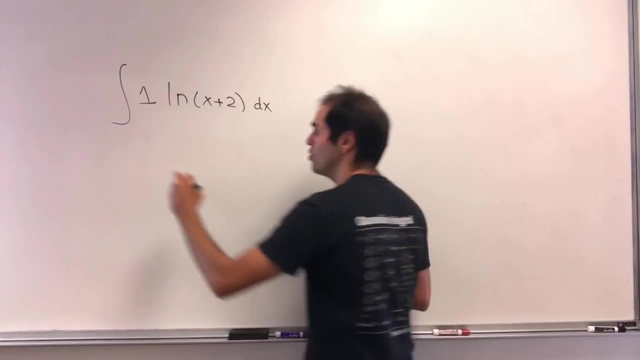 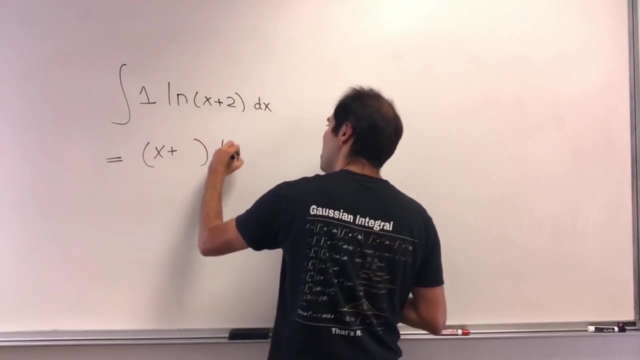 2.. So x plus 2.. x plus 2. dx. So here the standard trick is this is 1 times ln of x plus 2.. So this becomes an antiderivative of 1 is x, So x plus something, in this case ln of x plus 2 minus integral of x plus something. 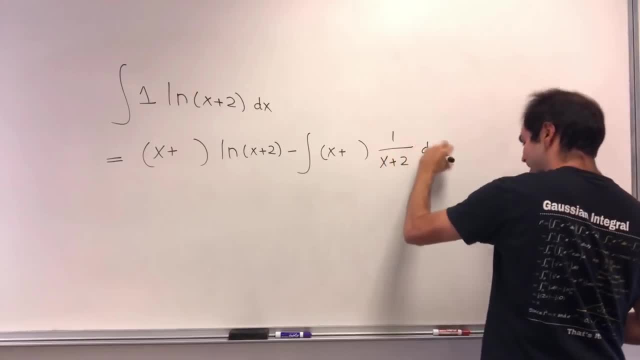 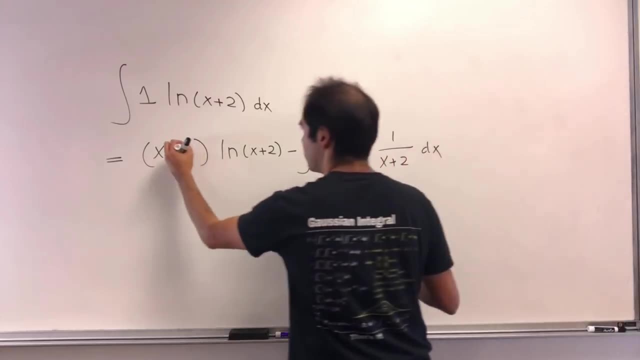 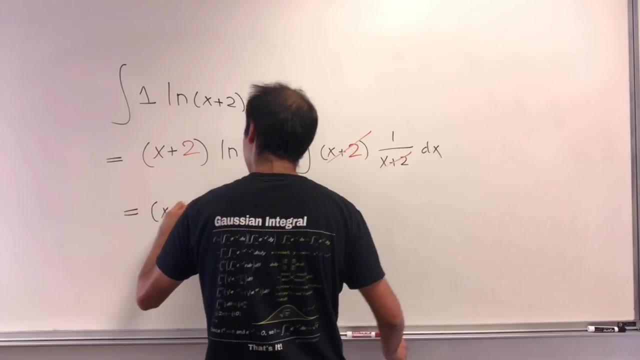 times 1 over x plus 2 dx. And then what is that? something We want to cancel out: the x plus 2.. So it becomes x plus 2.. And then, boom, boom, this cancels out And you're left with x plus 2, ln of x plus 2 minus integral of 1.. 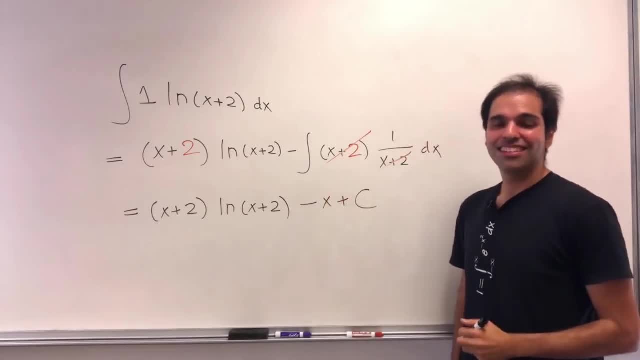 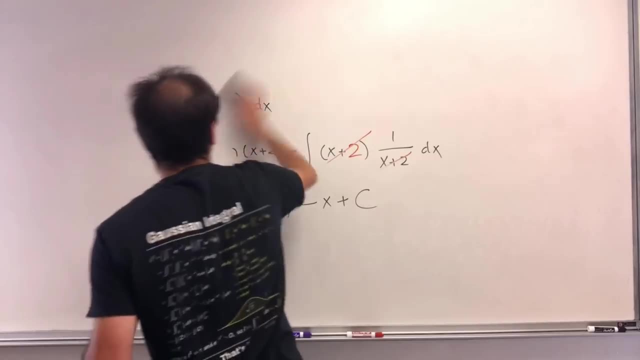 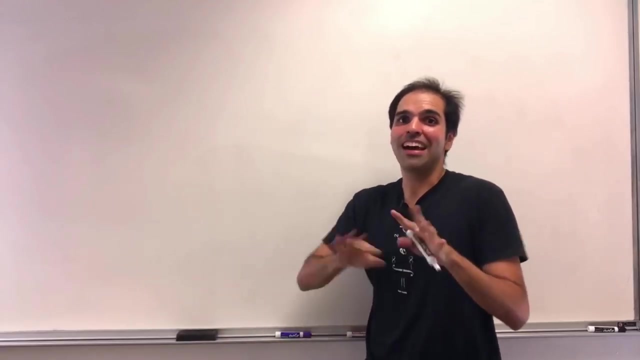 So minus x plus a constant, Isn't that nice? And last but not least, let's do one more example that's a bit more non-trivial. And in fact let's do what a calculus teacher does: Start with an easy problem and then make it spicy enough to become an exam prompt. 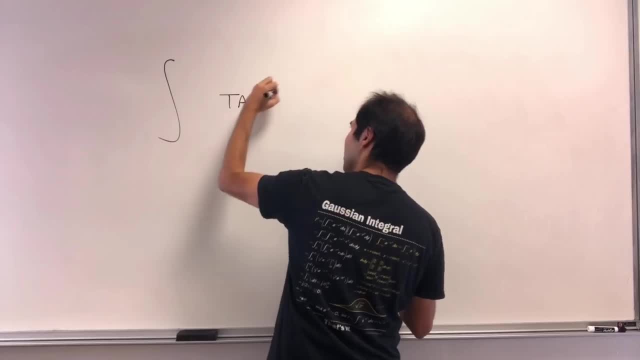 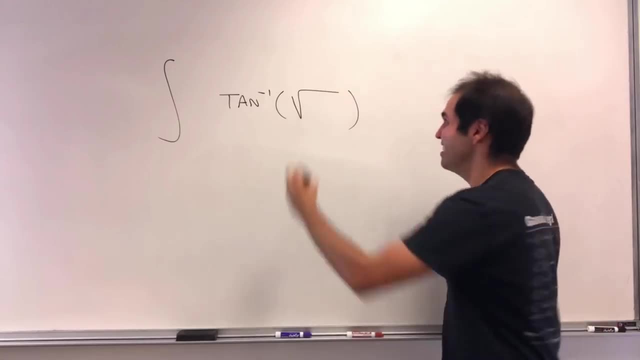 So how about we start with arctangent? But no, arctangent is too easy. Let's do arctangent of square root. Still too easy: Square root of x plus 1.. Ah, now even Drake would be happy. 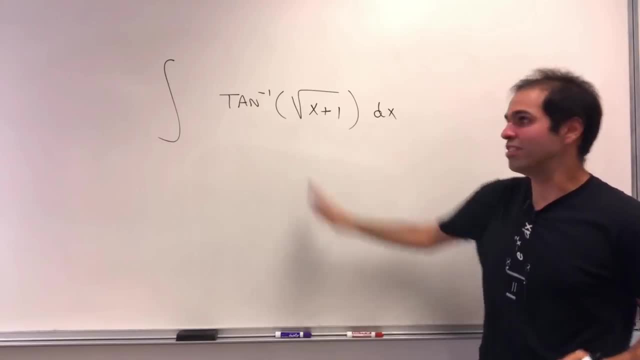 The x. OK, And again same spiel as before. This is 1 times arctangent of square root of x plus 1.. And again same spiel as before. This is 1 times arctangent of square root of x plus 1.. 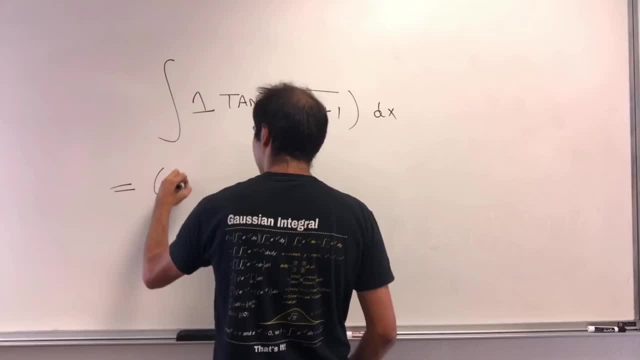 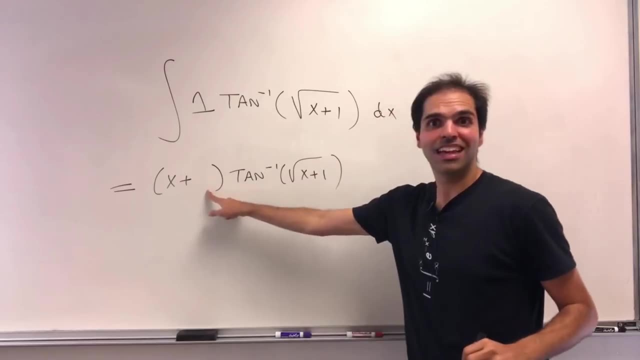 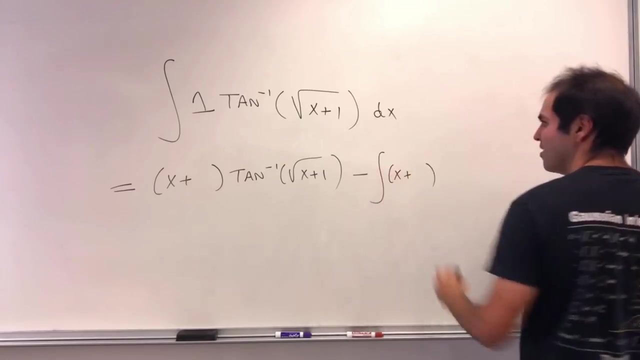 And this becomes now x plus something. times arctangent of square root of x plus 1.. And careful, the answer is not x plus 1. You actually have to work a bit harder. Minus integral of x plus something. Now for arctangent, let's use the chain loop. 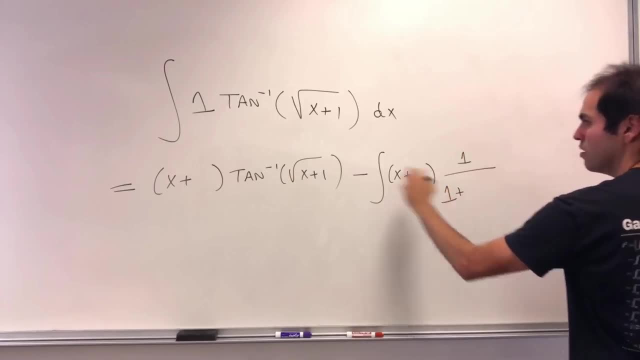 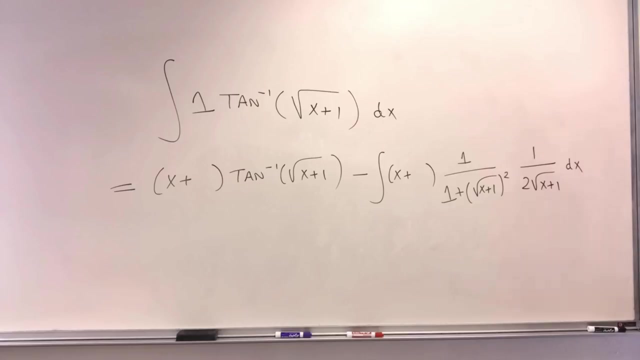 So this becomes 1 over 1 plus blast squared. So square root of x plus 1 squared Times derivative of a square root of x plus 1.. So 1 over 2 square root of x plus 1 dx. Okay. 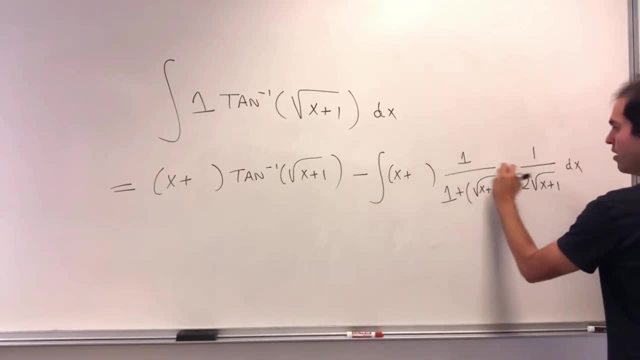 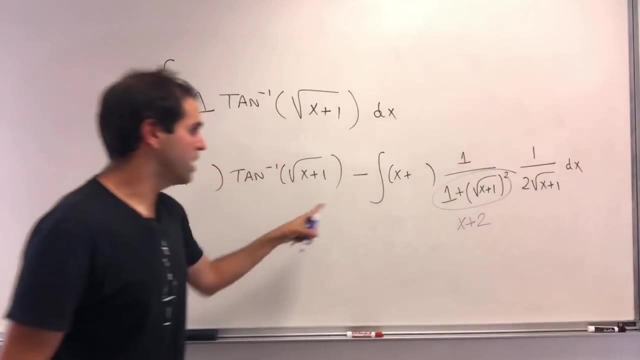 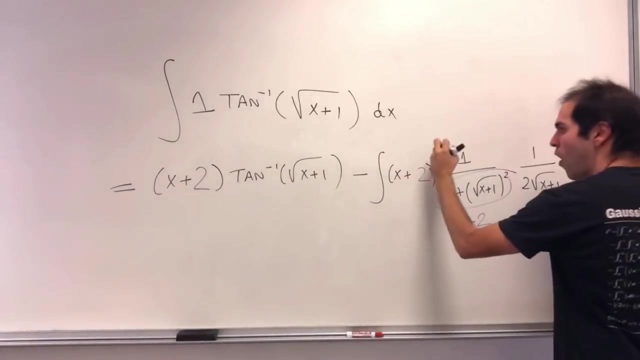 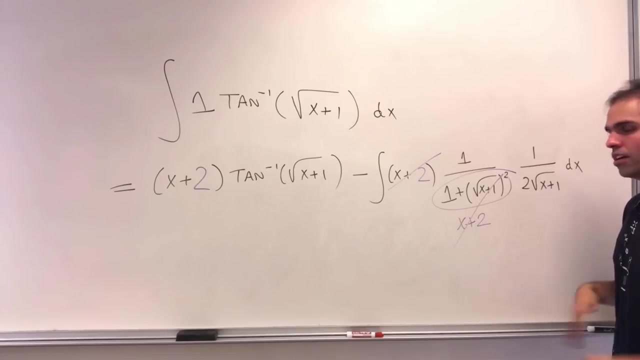 and here's the thing, Notice: the denominator now just becomes x plus 2.. So instead of choosing x plus 1, how about we choose x plus 2?? Then the nice thing again, the hard terms cancel out and you're just left with integral of 1 over 2, square root of x plus 1, which just becomes 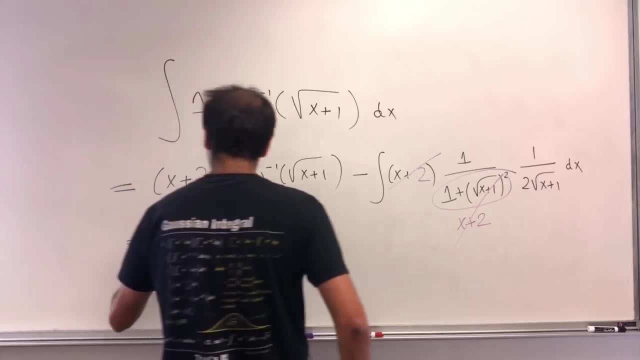 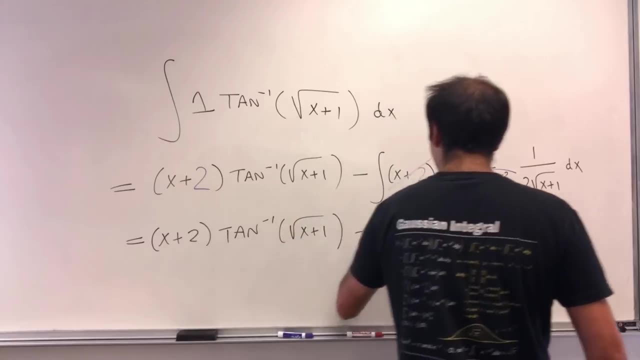 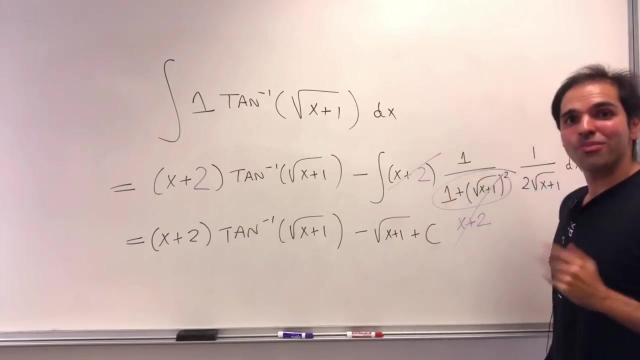 square root of x plus 1.. So in the end we get x plus 2 arctangent of square root of x plus 1 minus square root of x plus 1 plus a constant, And this is how we do it. All right, I hope you like this. If you want to see more math, 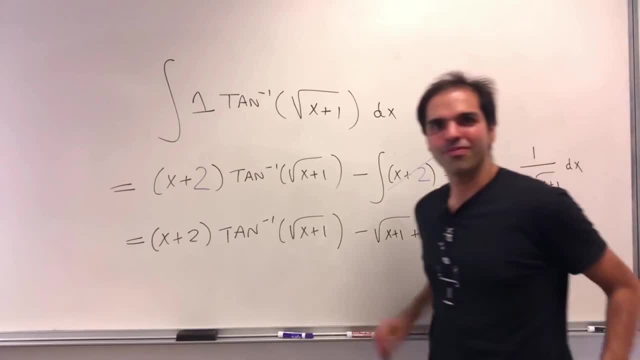 please make sure to subscribe to my channel. Thank you very much, Bye. 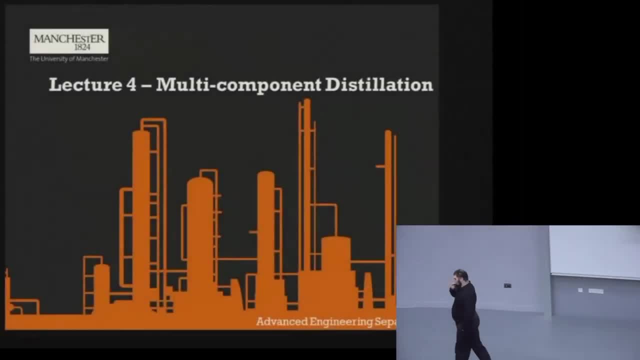 Okay, so today I want to move on to Chapter 3 in the handbooks, which is where we start to look at multi-component distillation. Okay, so we'll be building on what a lot of you did last year and looking at how we can think about distillation when we've got potentially 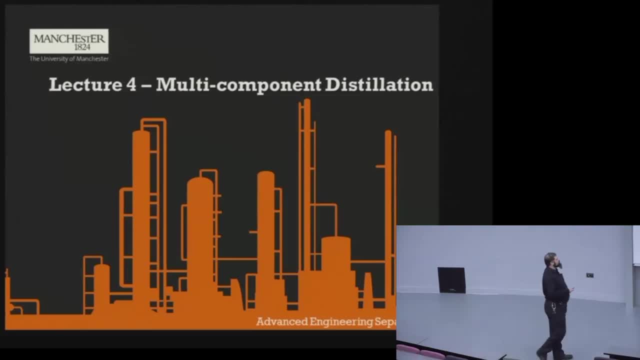 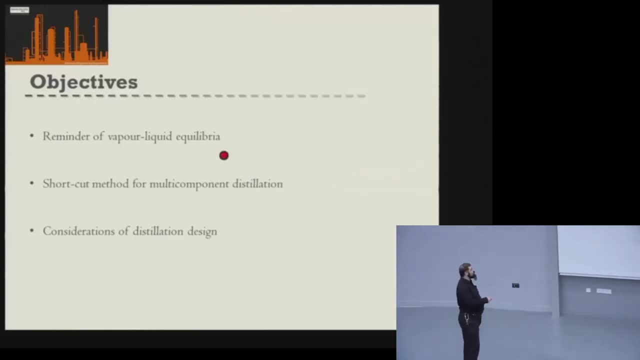 a lot more than two components. So I'll start off essentially with just a quick reminder for you of vapour-liquid equilibria, just so you remember what's important for this topic, And then we'll move on to thinking about how we can look at this multi-component.